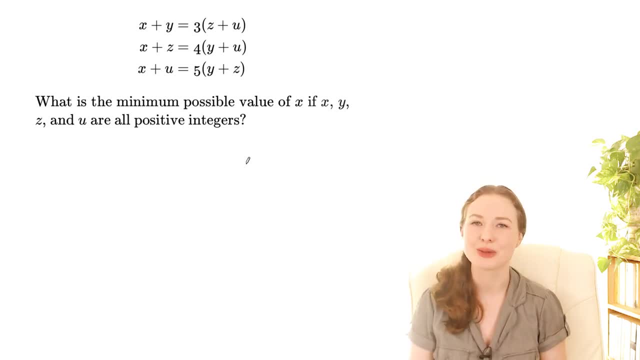 This question is from the 2007 Australian Mathematics Competition and 0% of students got this one right, although this one isn't multiple choice, which makes it harder. So we've got this system of equations and all the variables have to be positive integers, so whole numbers. 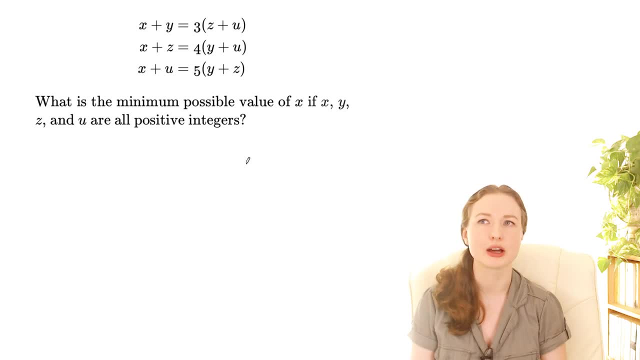 and we've got to work out the smallest possible value of x. So there's going to be like multiple solutions, but we want to work out the smallest value that x can take. So you might like to pause the video here and give that question a go. Now, personally, what I like to do where you've 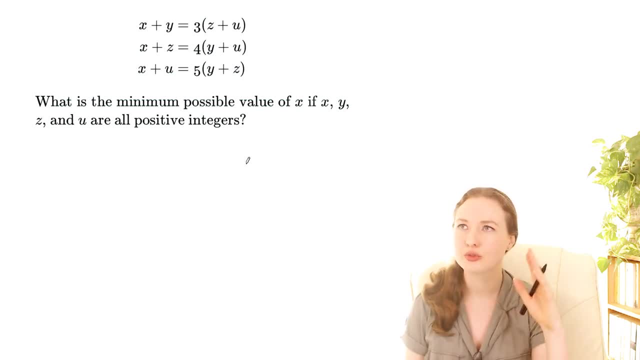 got systems of equations like this is just move all the variables onto one side. That's kind of like the standard linear algebra way of handling these things. So we could say like with that first one I might just shift these over to the left. I'm just sort of more comfortable with it. 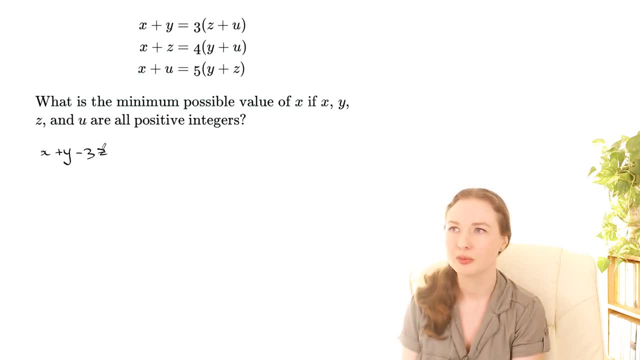 that way, So 3z. but in mathematics we always put a line through the z's so they don't look like twos. So that's, I'll call that equation 1, and what you also want to do is keep all the variables in the. 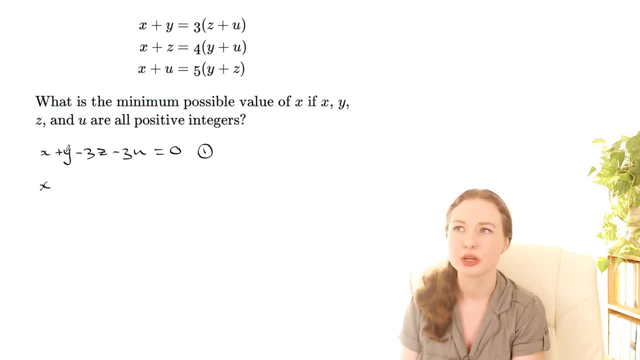 same order. So I don't want to say x plus z, because up here I had y as the next variable. so when I shift this across I'm going to have x minus 4y and then plus the z minus 4u- let's call that equation 2, and then with this one we've got x minus 5y minus 5z plus u equals 0.. 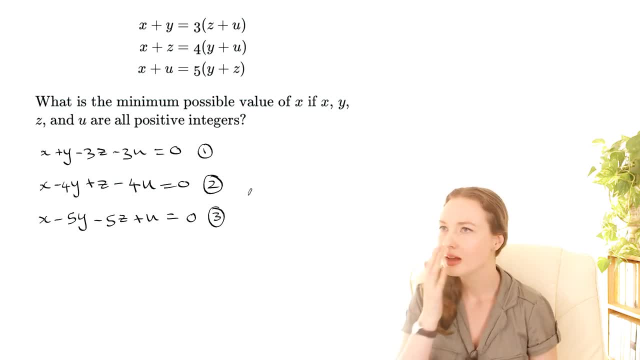 I'm going to call that equation 3.. Now, kind of the. the easiest way to eliminate things would be to get rid of x's because, like, the coefficients are all 1, but since we're trying to find the minimum possible value of x, what I'm going to do is eliminate something else. 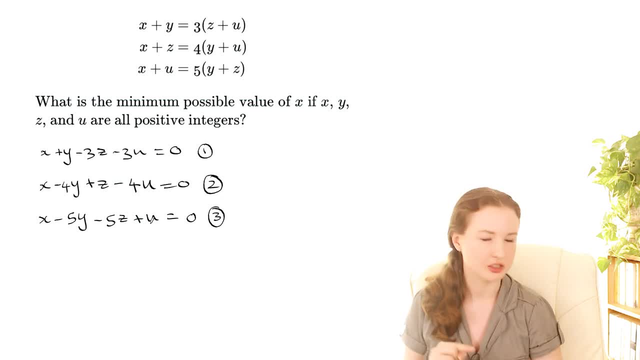 instead, In the solutions they actually did eliminate x, but I found that way a bit confusing, because what they did was they they found like the minimum solutions for I don't know, like y and z or something, and then they just said, okay, well, therefore, the minimum value of x will be when? 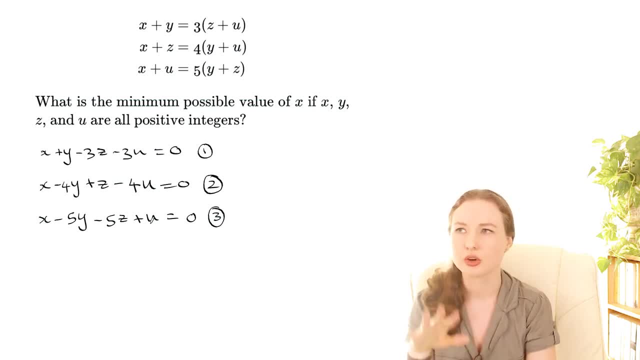 we use those values, which I didn't think was obvious. So I want to just get rid of everything but x. Alright, so what I'm going to do is notice that the coefficient here is 1, so that one's going to be a good one to use to eliminate the u's in the other equations, So like if I multiply. 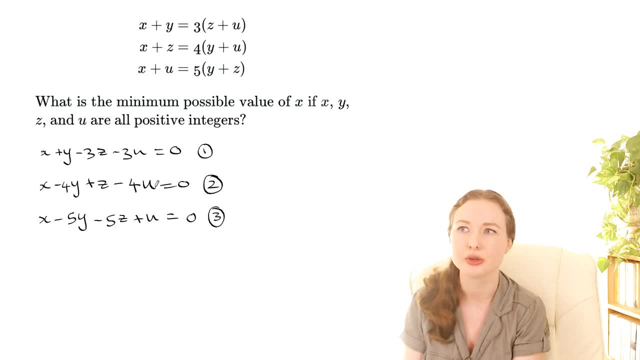 this one by 4 and add it to this one, that's going to get rid of the u's. or if I multiply it by 3 and add it to that one, it's going to get rid of the u's there. So let's try that, let's go. equation 1: 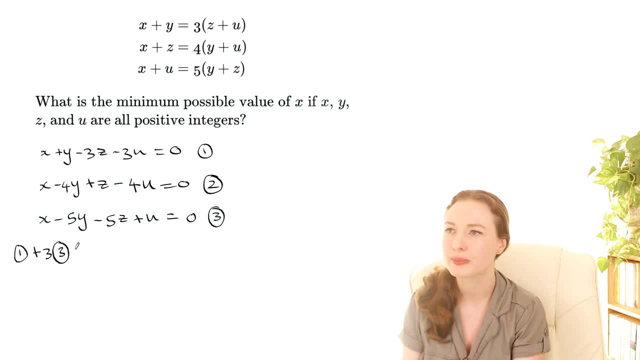 plus 3 times equation 3 and see what happens. So 1 of that and 3 of that make 4x, and then we'll have so 1y and negative 15, negative 14y, and then we'll have 1 of that, so negative 3 minus 15, negative 18z. The? u's will cancel. 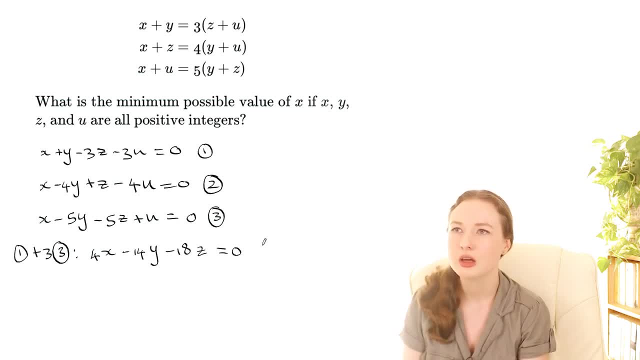 and then we've got a 0 on the right hand side. I'm going to call that equation 4.. Now, if any of you haven't done linear algebra before, I just might go on a tangent here about the history of this stuff. you might see how irritating it is to keep having to write, you know. 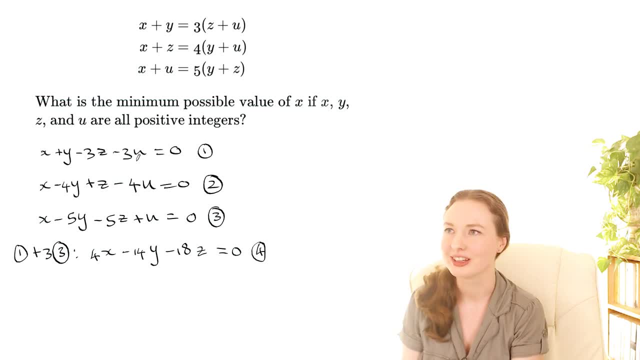 the x's and y's and z's and u's, and think you know, wouldn't it be nice if we could just say, okay, that coefficient is 1, and then that coefficient is 1, and then that one's negative 3, and that one's negative 3, and so on and so on? 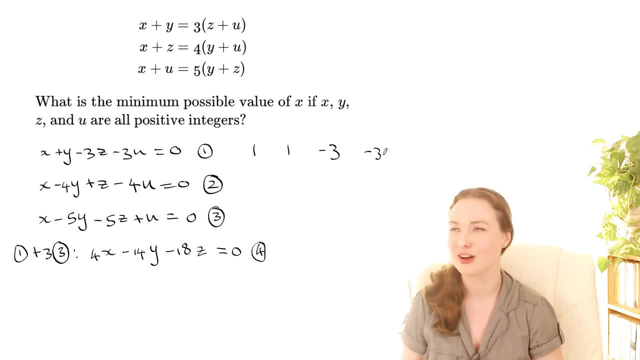 Wouldn't that be simpler? Well, that's exactly what the Chinese thought in, I think it was, the Nine Chapters of the Mathematical Art, which was one of the first examples of matrices being used, which just sort of simplifies this whole thing, Anyway, but 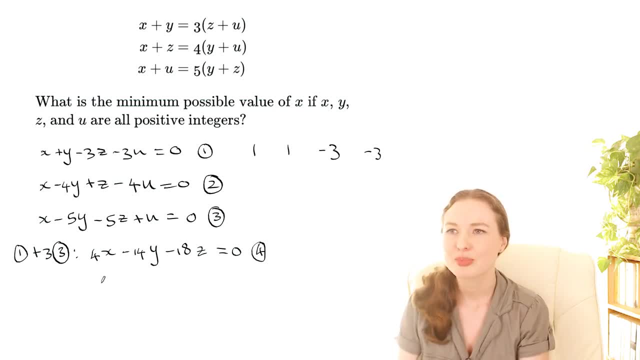 I'm not going to use like matrix notation here. Okay, so that's equation 4,. we've gotten rid of the? u. Let's do the same thing with this equation. So I'm going to take equation 2 and add 4 times equation 3, because that's going to get rid of the u's. So we've got that. 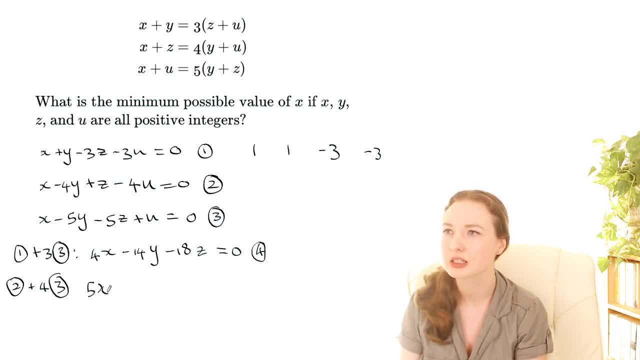 plus 4, so that's 5x negative, 4 minus 20, negative 24y, and then we'll have 1 minus 20, negative 19z, and then the? u's will cancel and we get 0.. Let's call that equation. 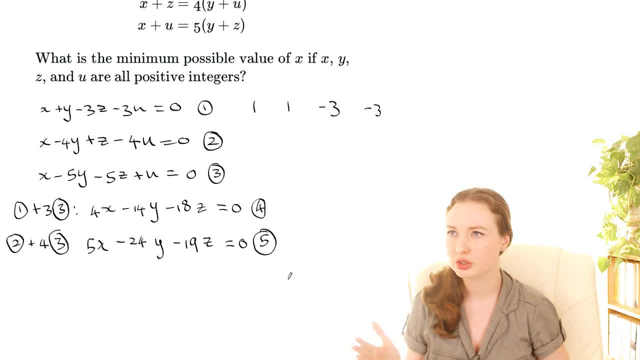 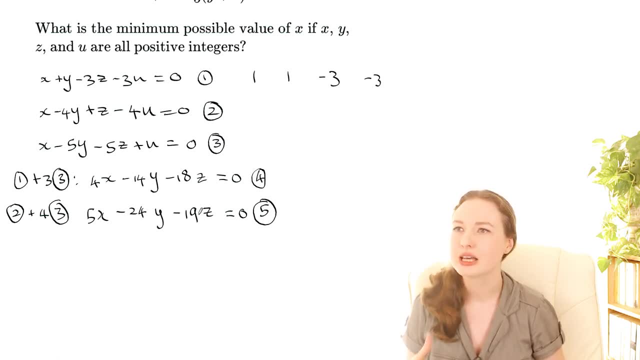 5. Now we need to eliminate either y or z from these equations. The z's are a bit annoying because 19 and 18, that's going to be irritating. to multiply everything by but the 14 and the 24 here we might be able to find like a: 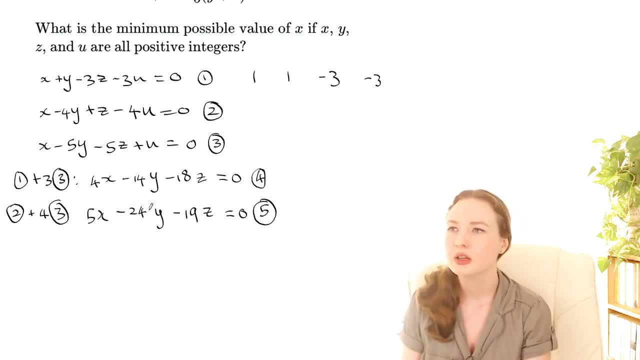 lower LCM, since they're both. even So, if you, the way that I think about it is that the 14 is 2 by 7 and the 24 is 2 by 12, so, if I like, we don't want to repeat the. 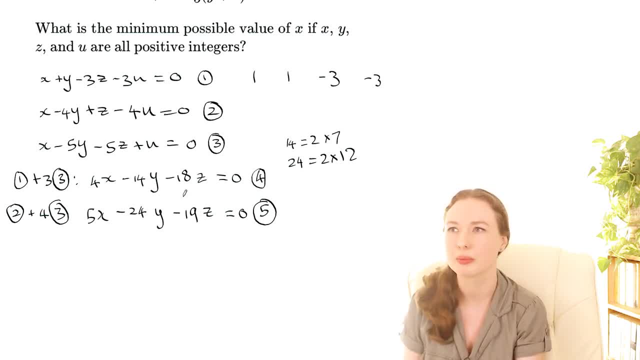 two, like I don't want to just multiply this by 14 and multiply that by 24, because then you're sort of doubling up on the two which you don't need to. What we could do is just multiply this one by 7 and this one by 12, and then that'll. 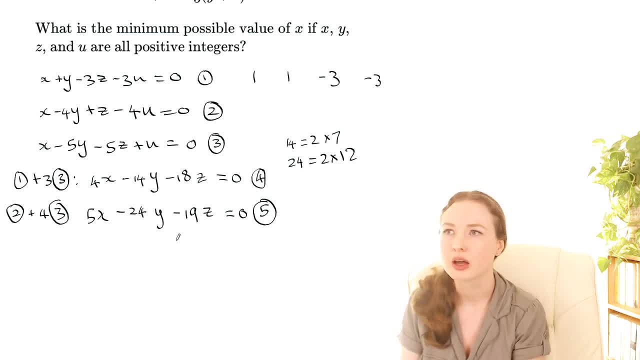 the y's will cancel out. So let's do that. So I want 12 times this one, so 12 times equation 4, and then minus 7 times equation 5. And that should get rid of the y's. Okay, so we've got 12 times this. 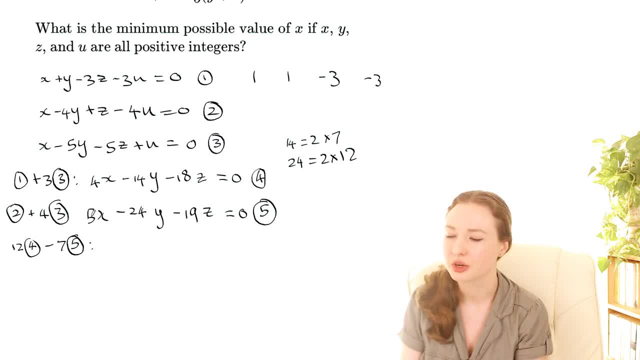 so 48 minus 7 times that, so 35. So 48 minus 35 is 13x. Those will cancel. I'm going to do that And then so we're not allowed calculators for this exam, so I'll just 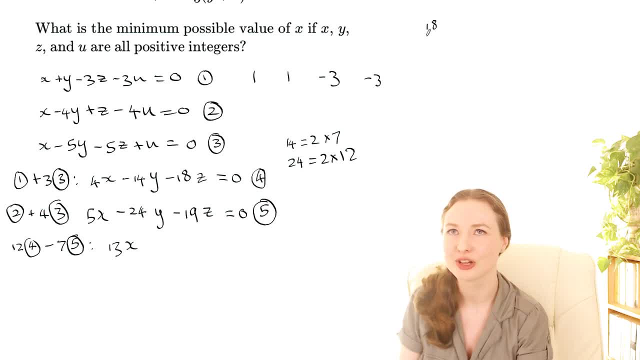 have to do 12 by 18.. I don't know my 12 times tables, So I just have to do it this way. I feel like I've made a mistake there. Yes, I definitely have. That was meant to be a 1.. I'm trying to talk and think at the same time. It's not good. 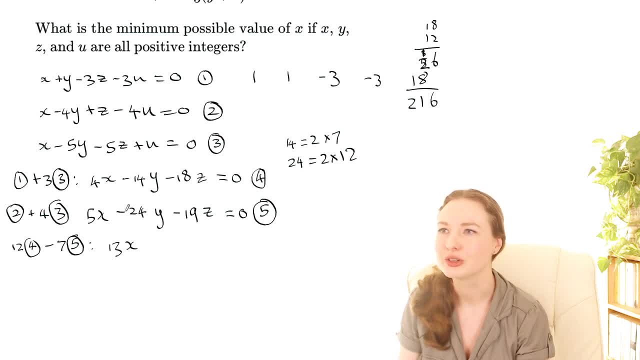 Okay, 216.. And then if we do 7 times the 24. then we no, We're doing 7 times 19.. Sorry, 7 times 19.. 63.. 7 times 1., 7. and that makes 13.. So we've got that one's. 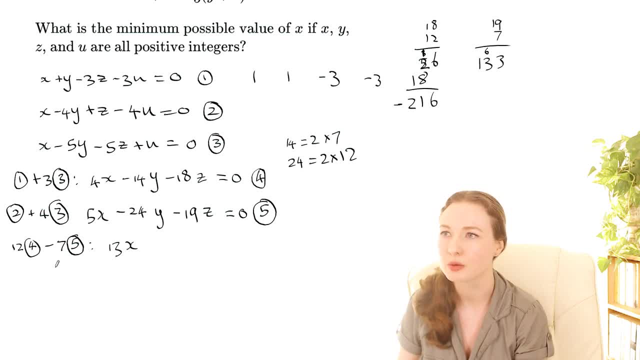 actually negative, because that's a negative 18, that one becomes positive because we're subtracting that. so we want like 133 minus 216, I'll just do 216 minus 133 over here, so 83,. so we'll get, except that it's. 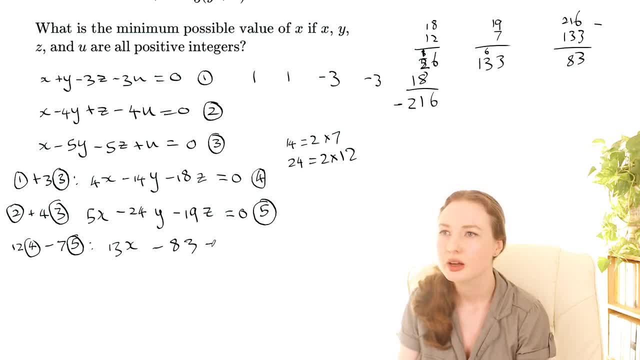 negative 83, because that was the one that was negative. Okay, and then what I might do is just shift that over to the right. So we've got 13x equals 83z. Now let's think about the fact that they're positive integers. So if you've done Diophantine equations before this, 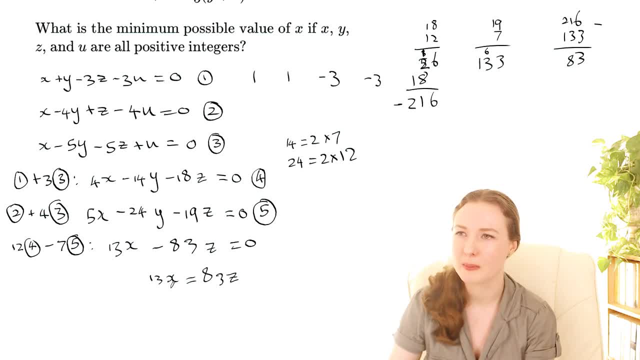 might be easier for you. but the kind of idea is that because over here we've got 13 times an integer, it's right in the interval where b and 1 is the next integer, so we're square 3 and Negro. So 15 times these亨's quiere 33.. Now let's shift over to the right, so we got 13x equals 83, that's the area atiendo the positive part. then we just shift the positive part so we got 13x dakos becoming~~ 13x eqademумou. Now let's think about the fact that they positive integers. So if you've done Diophantine equations before, this might be easier for you. but the kind of idea is the because over here we've got your 13 times and 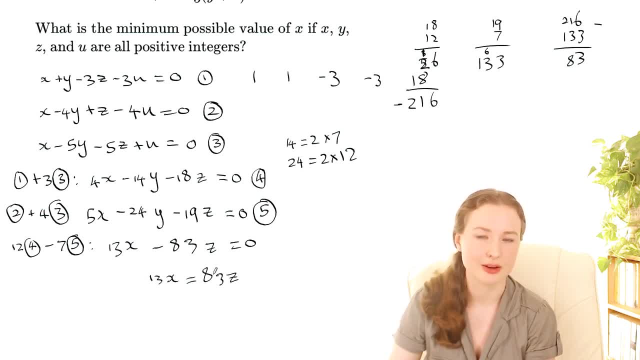 integer, that means this is a multiple of 13,. right, So this has to be a multiple of 13.. Now, 13 doesn't go into 83 and, like they don't have any common factors, this is actually prime. so that means that z has to be a multiple of 13.. And similarly,